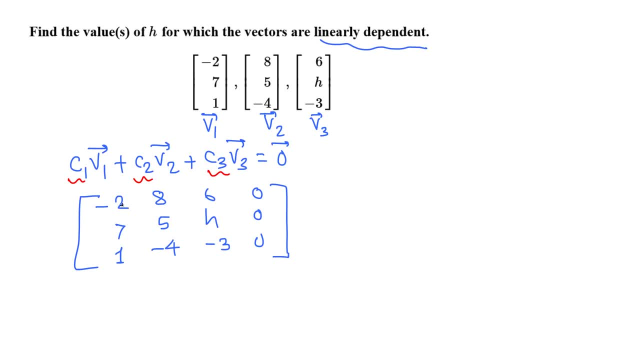 okay, that means pivot in the first, very first. then we make zero, zero, zero, zero. pivot 0, okay, negative 2. look at in r3 we got 1, so we can swap r1 and r3. okay, let's swap r1 and r3, so r1, r3 becomes r1, 1, negative, 4, negative 3, 0, r2 stays the. 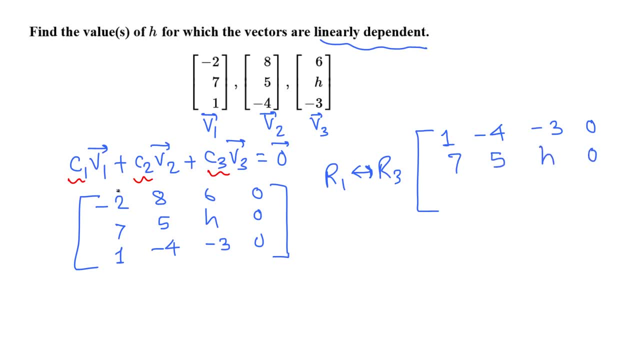 same: 7, 5, 8, 0 and it is negative: 2, 8, 6, 0. okay, row reduce means we want to make this 0, we want to make this 0, we want to make this 0. okay, and this will be pivot 1. I mean 5. that should be pivot, it might. 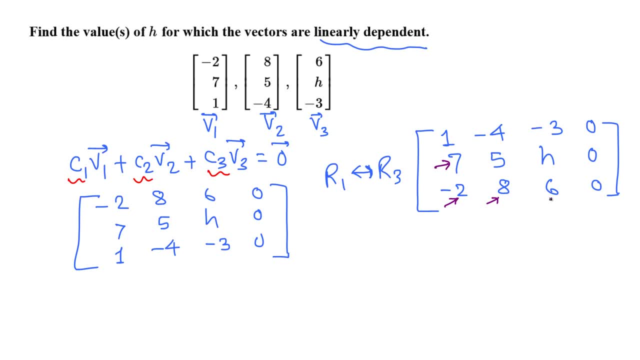 change 6. that should be pivot location, but it might change, okay. so looking at the, so I want we can do two things at the same time. let's make this zero, so for that we can r2, so to make zero, so r2 plus 7 plus negative 7, 7, r1, okay that. 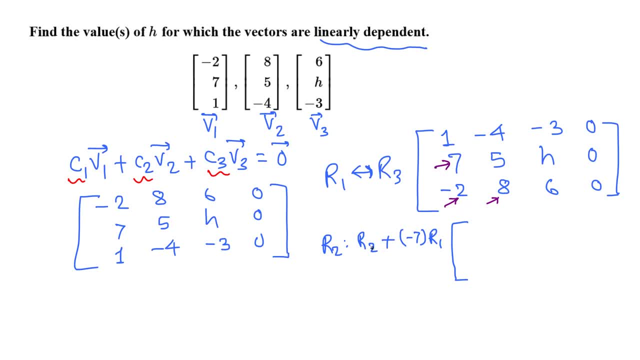 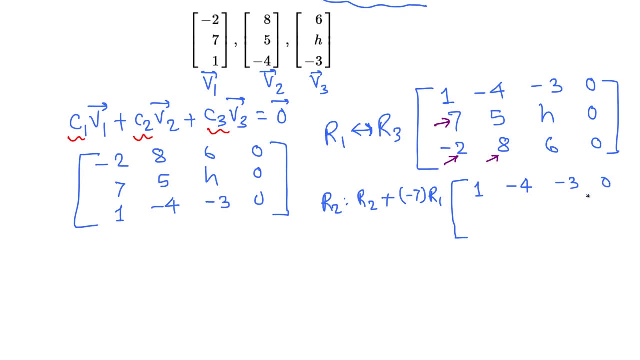 makes this zero, and we can make this zero as well. so here: 1 negative, 4 negative, 4 negative, 3, 0. now, 7 times negative, 7 is 0, 5 plus negative. 7 times negative: 4, 28, 5 plus 28, 33. okay, here is H plus 21. this is zero. now we can make. 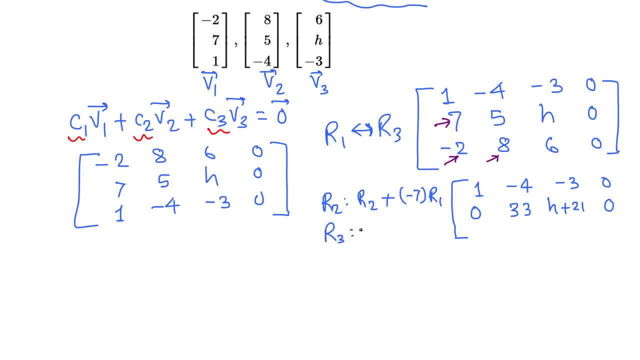 this 0 as well. now we can make this 0 as well. that means r3, r3 plus negative 2. here is 2 times r1. now, if you, if you look at closely- 1 negative, 4 negative, 3, 0. the third row is just constant multiple of. 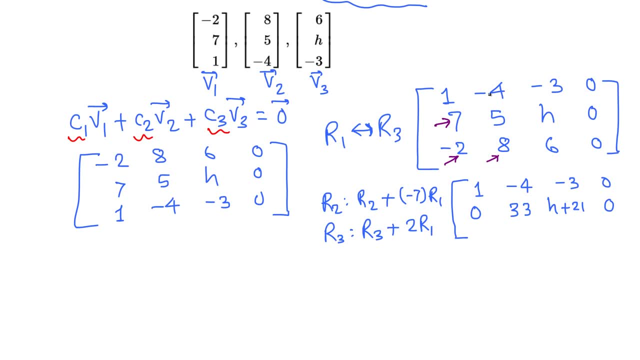 first row because 1 times negative 2 is negative, 2 negative. 4 times negative 2 is 8 negative. 3 times negative 2 is positive 6. so we don't have to even write anything, because we saw that these two columns are just constant. 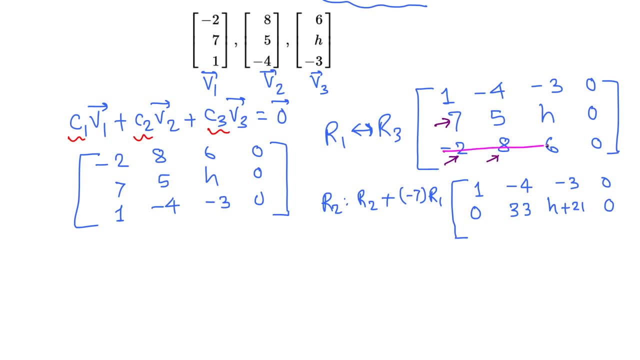 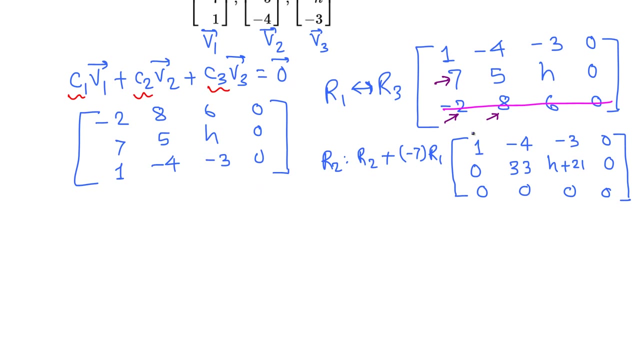 multiple of each other. so we can pretty much say, oh, this is all zero, okay, and we can just write 0, 0, 0, 0. now what can be said about this system here now? so this, if we try to solve this one is: first: column is for c1. 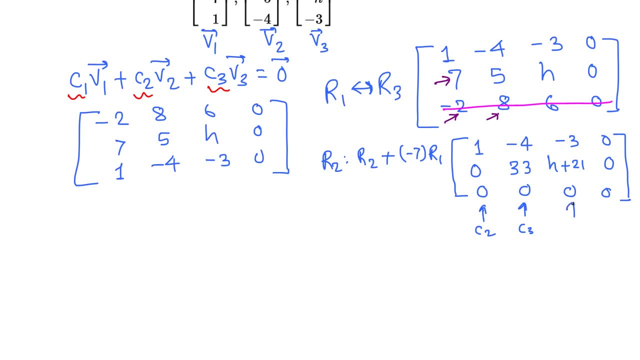 this is for c2 and it is for r3. this is for c3 and there is no pivot in the last, in the last column. that means we have solution. okay, there is no pivot in the last column means we have solution. the system is consistent and, at the same time, there is no pivot in the 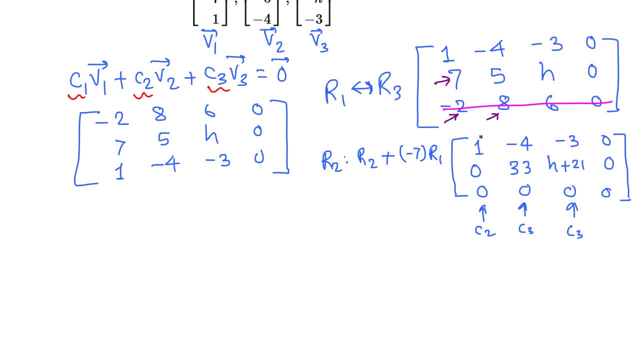 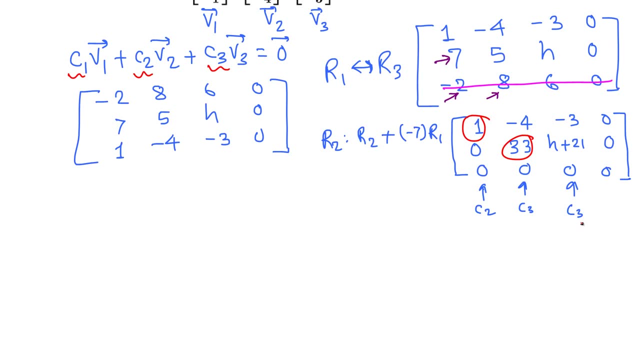 third column as well. we got pivot here and here, but there is no pivot. that means this c3 is a free variable. okay, this is free variable. free variable means we always get non-trivial solution. in fact, we get infinitely many solutions. okay, Whenever there is a consistent system, we 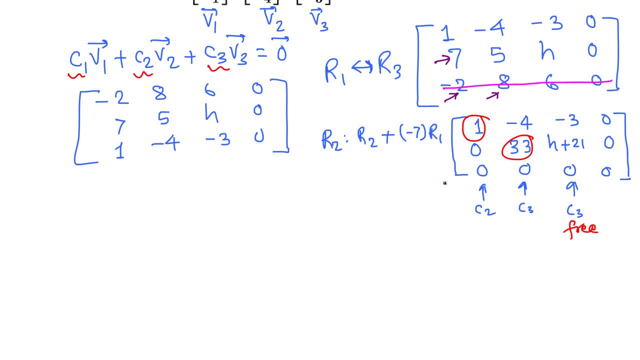 have two cases: one solution, same as unique solution, or infinitely many solutions. here we got a free variable. free variable means we getano in tomb position and no pivot in the next column as well. So this is another internet or eucza ares- Someone is following here- so you can simply click a patient we on to backup the system. So here you have to just type anywhere you do. things is a consistent system. we have two cases: one solution- yes, unique solution, or infinite solutions. here we got a free variable. free variable means we get 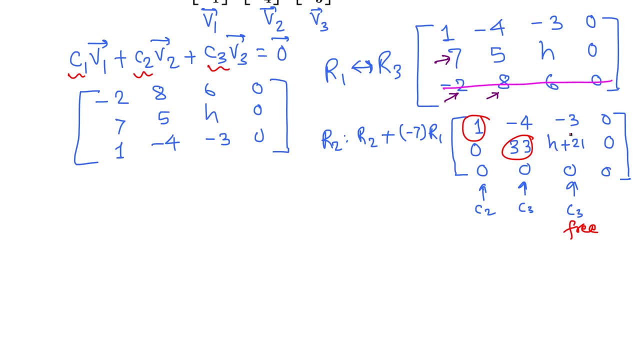 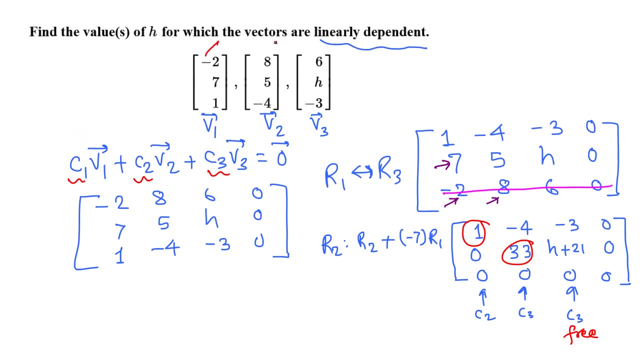 infinitely many solutions. regardless the value of h, regardless the value of h, we get infinitely many solutions. That means these three, the given vectors. okay, these three are linearly dependent, for any value of h doesn't matter, h can be negative, 21, that's fine, or any other values, because the third variable is: